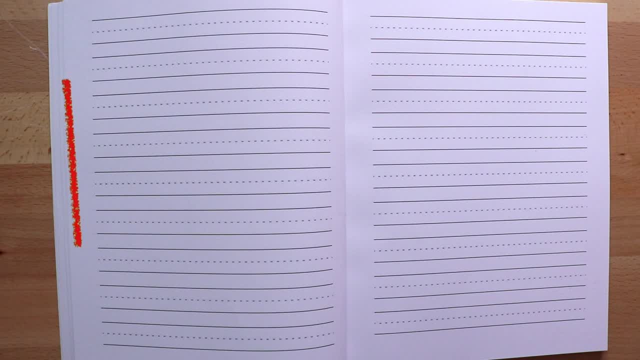 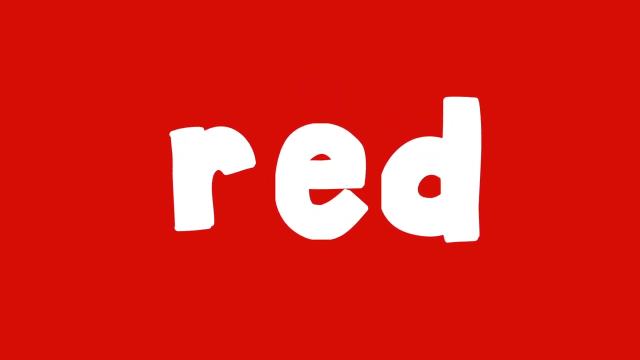 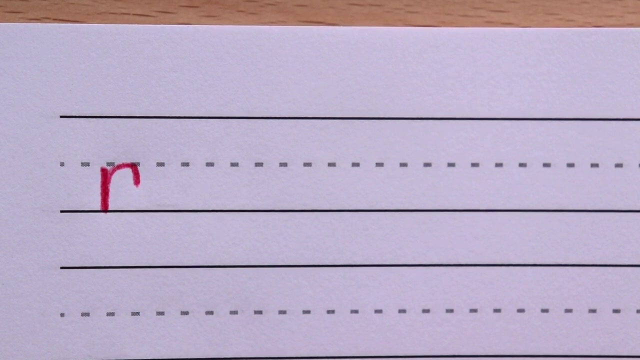 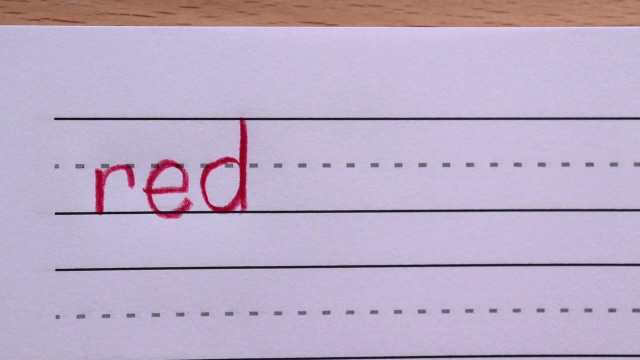 When we write, we use straight lines, curved lines, circles and sometimes dots. Let's try Red R E D, Red R, Boing E, Boing D. Now let's make a color spell. 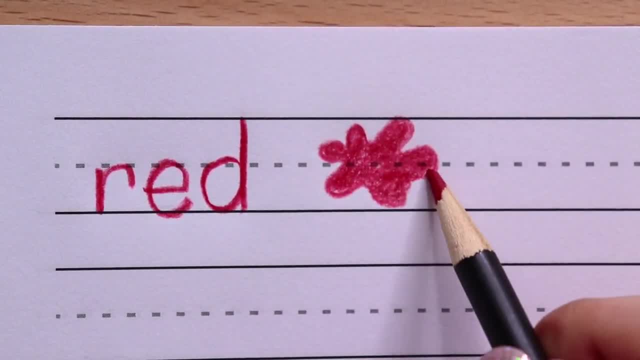 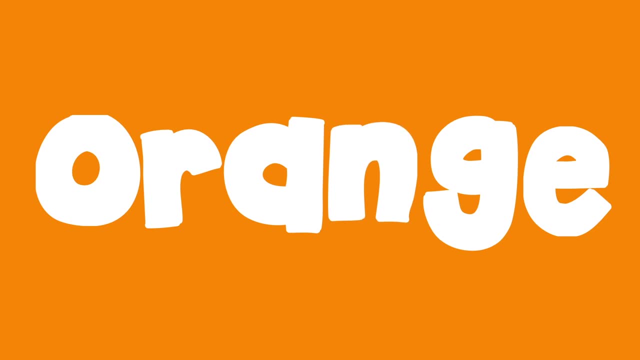 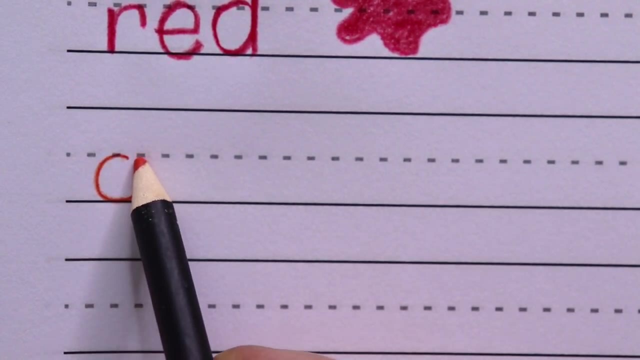 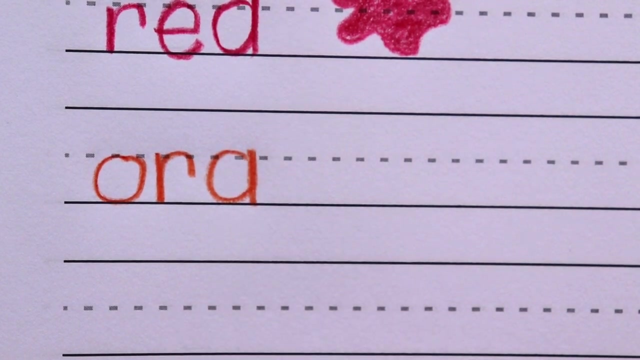 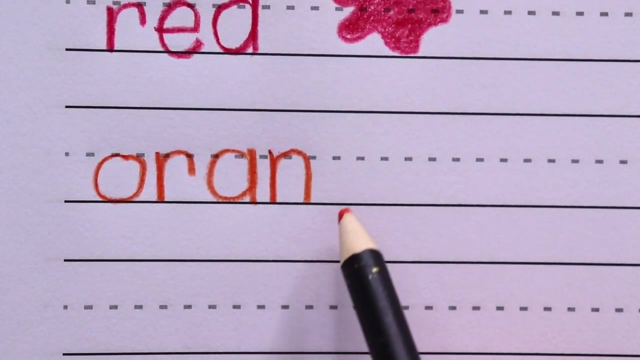 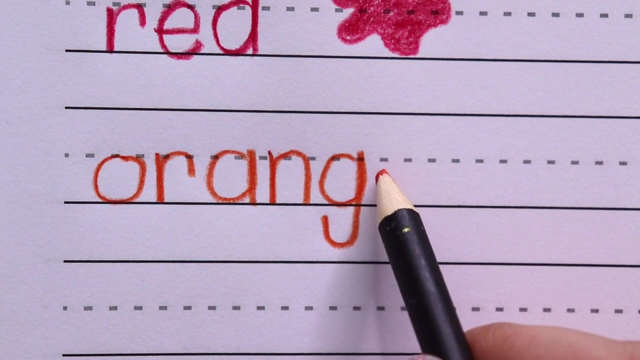 Splat for fun, Color color color. splat Orange O-r-a-n-g-e Orange O R Boing A Gosh S S S N Boing G, Boing E Boing Now. color, color color. 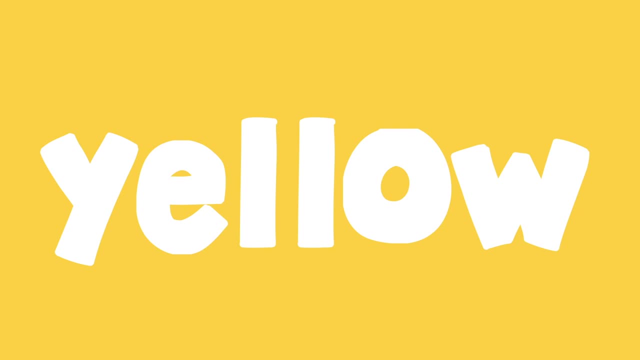 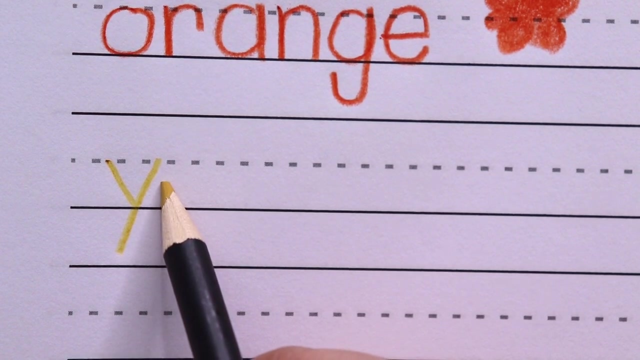 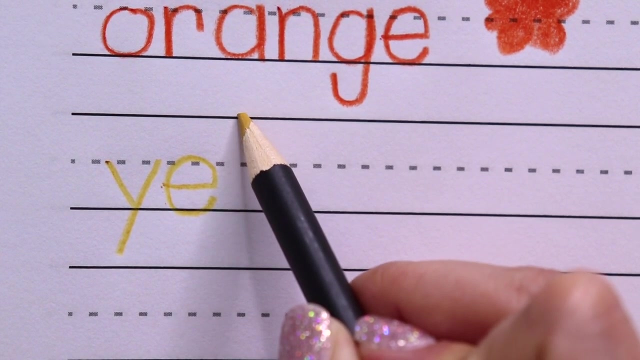 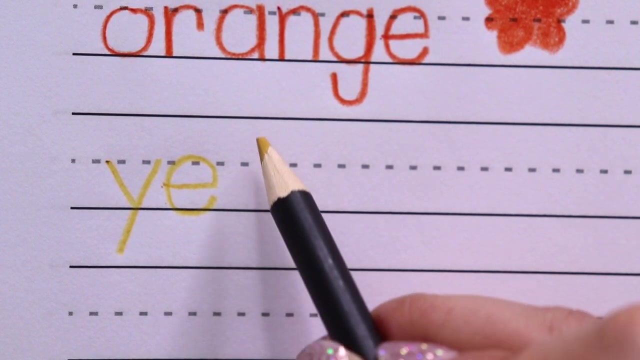 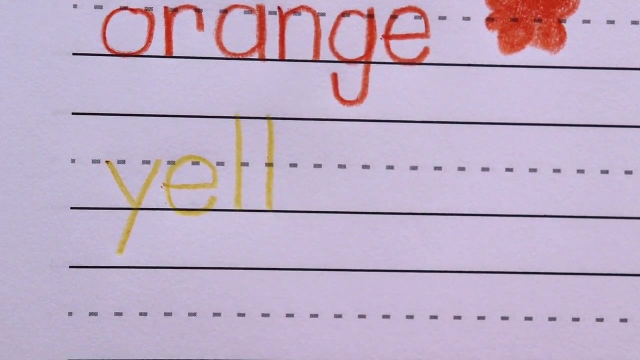 Splat Yellow Y-E-L-L-O-W. Yellow Y E Boing L L is a tall letter. Let's make sure it touches the top all the way down to the bottom line. Ready L O W, Now color, color, color. 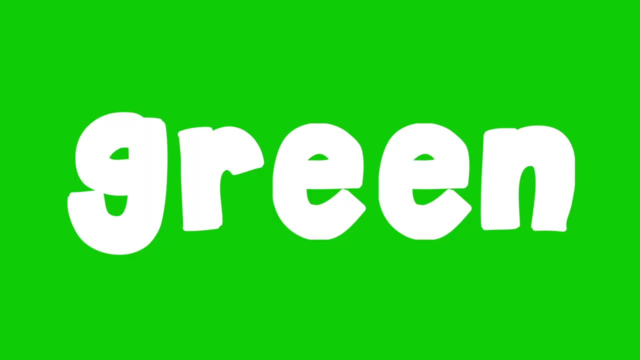 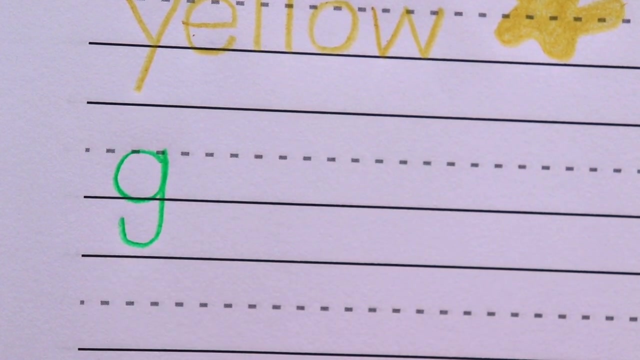 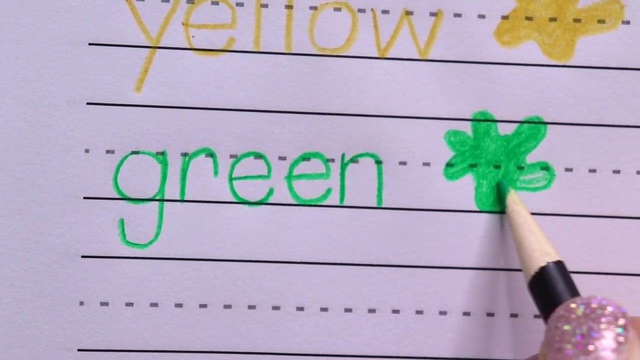 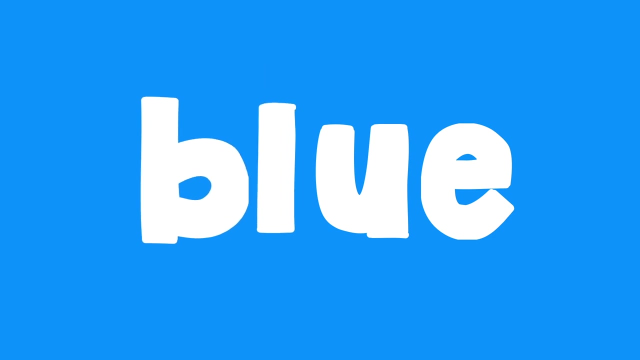 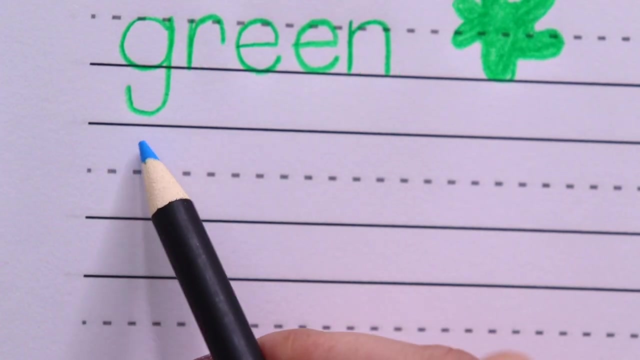 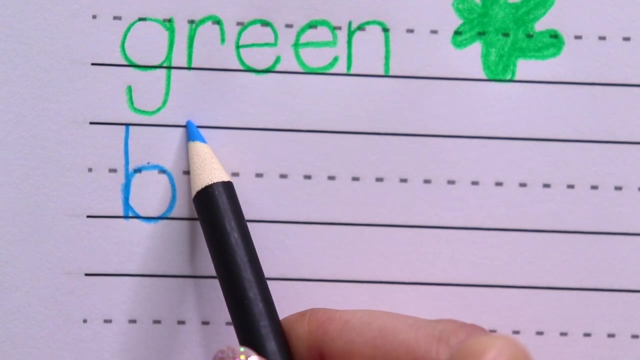 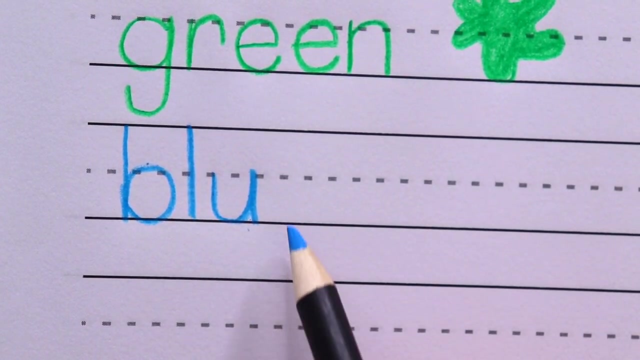 Splat Green G-R-E-E-N Green G Boing R, Boing E, Boing E, Boing N, Boing Now, color color color. Splat Blue B-L-U-E Blue B? L? U, Boing E. 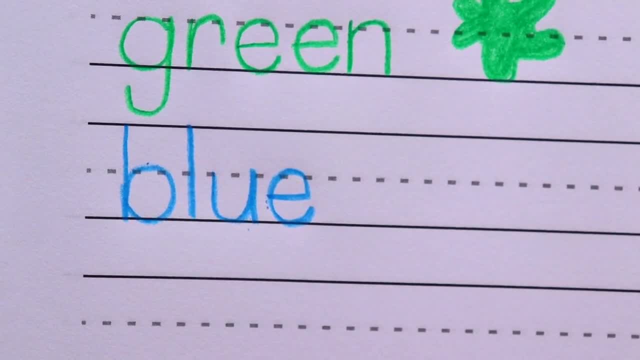 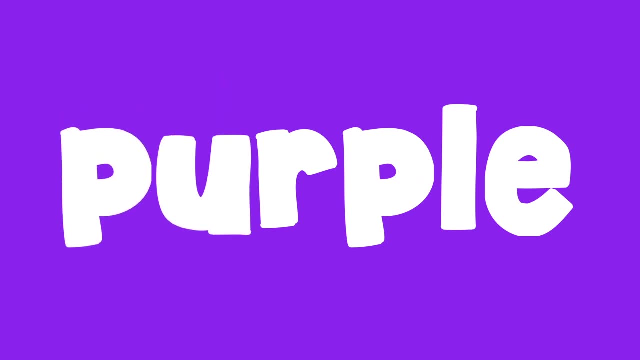 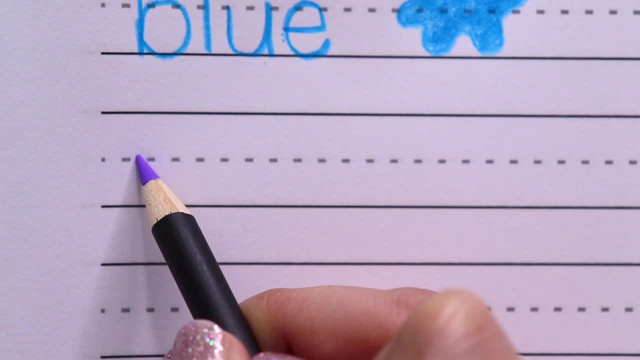 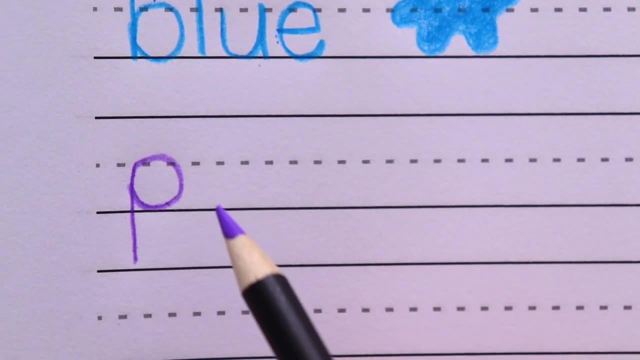 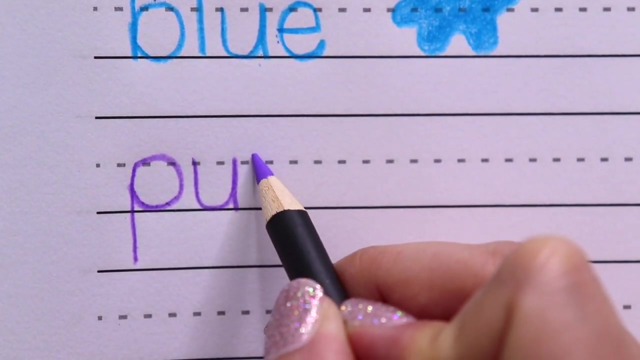 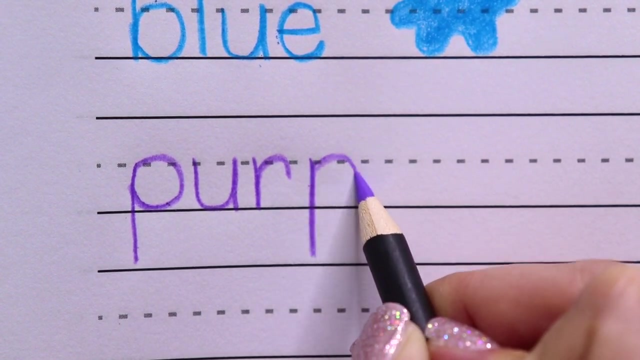 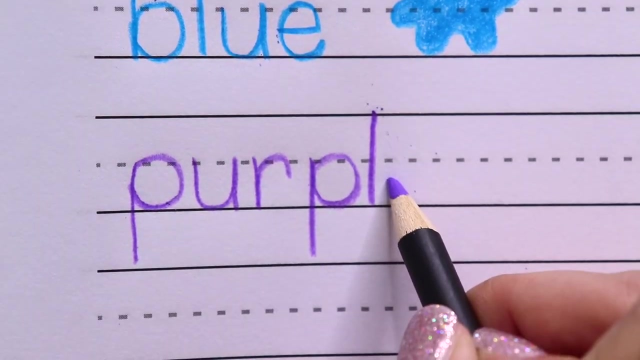 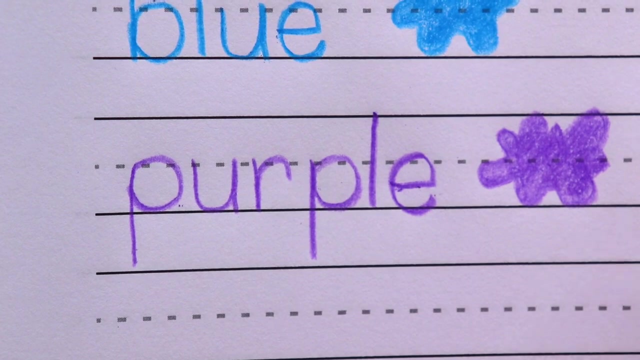 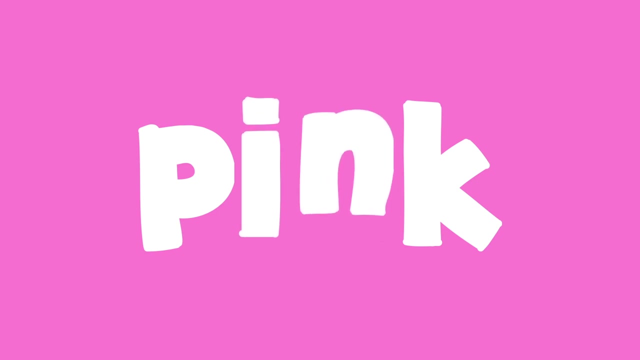 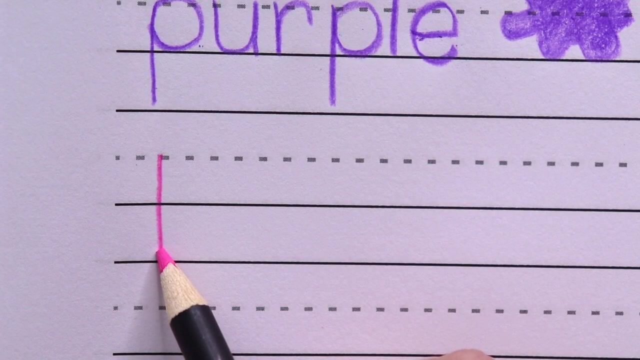 Purple P Under the lower line: U Boing R Boing. Boing P L E Boing Color color color Splat Pink P I N K. Pink P I.